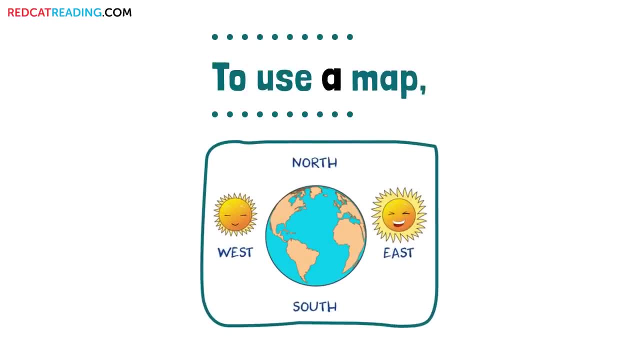 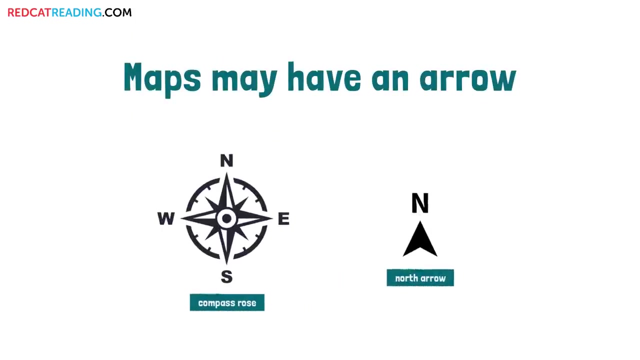 Parts of a map. To use a map, first learn the four directions: North is the direction of the North Pole, South is the direction of the South Pole, East is where the sun rises And west is where the sun sets. Maps may have different directions. 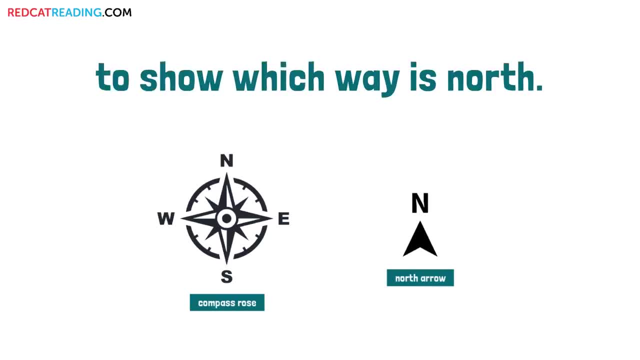 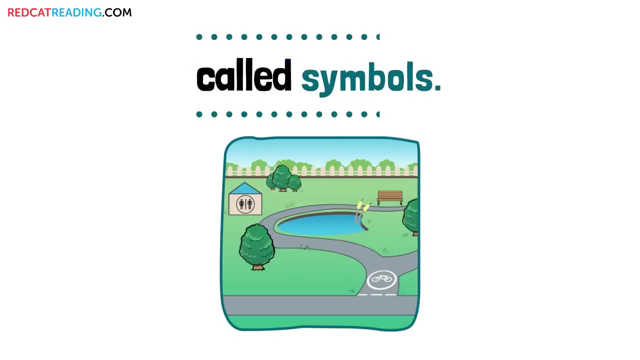 They may have an arrow and the letter N to show which way is north. They may instead have a compass rose with all four directions. Maps may also have little drawings called symbols. A little bike may mark a bike path. Cities and parks use a symbol to help people find bathrooms. 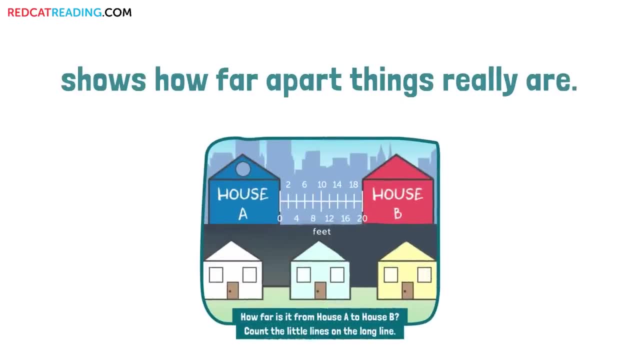 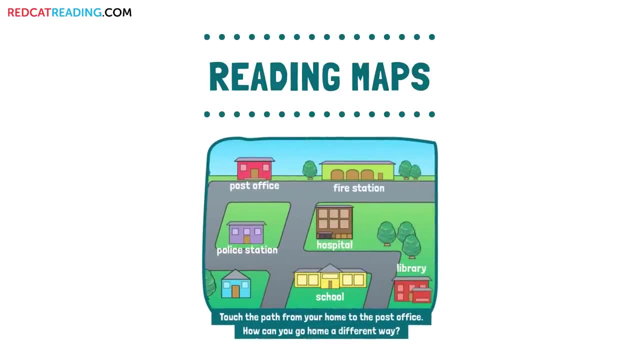 Maps may have a map on the side. A scale on a map shows how far apart things really are. Mapping maps: Look at the map on this page. Pretend you live in the blue house. Walk your fingers from your house to the library. 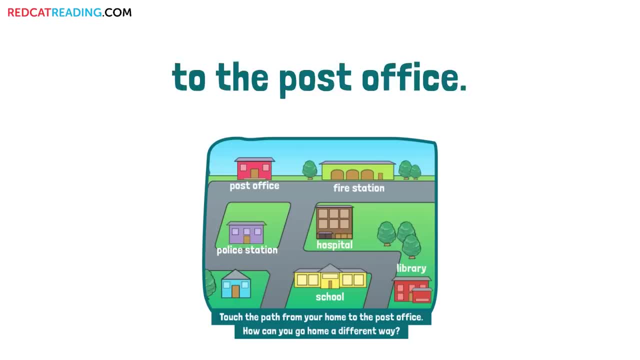 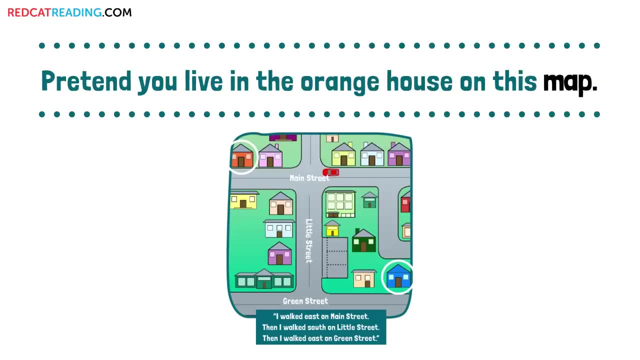 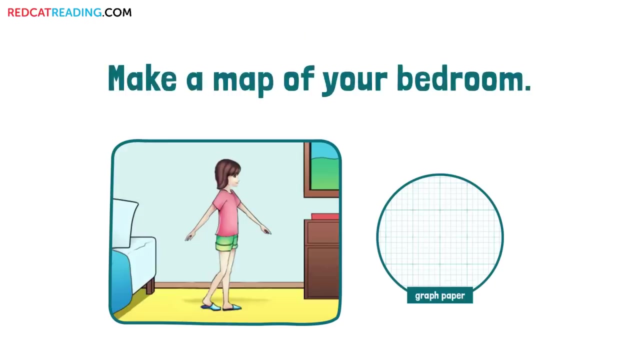 Now walk your fingers from the library to the post office. Pretend you live in the orange house on this map. Walk your fingers to the blue house. Use words to tell someone how you got there. Making maps: Make a map of your bedroom. 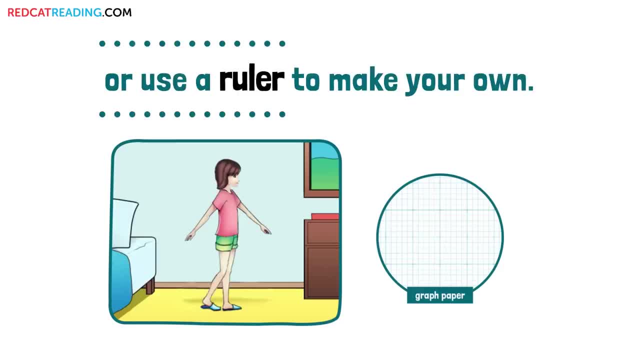 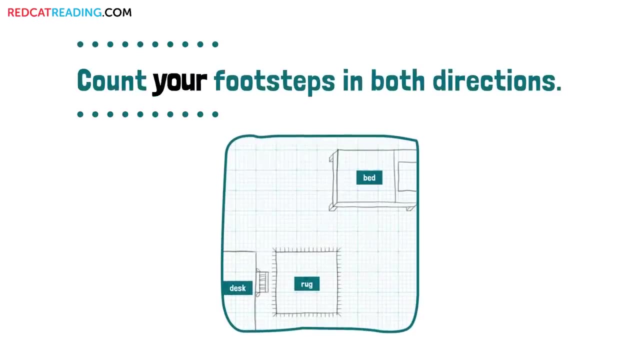 Start with some graph paper or use a ruler to make your own. Measure the room with your footsteps. Each footstep equals one square on the graph paper. Count your footsteps in both directions. Then count the same number of squares on the paper. 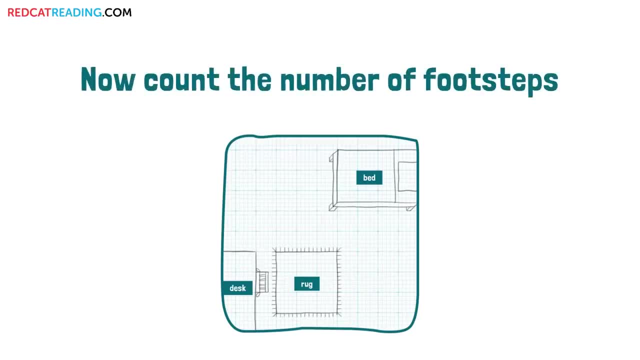 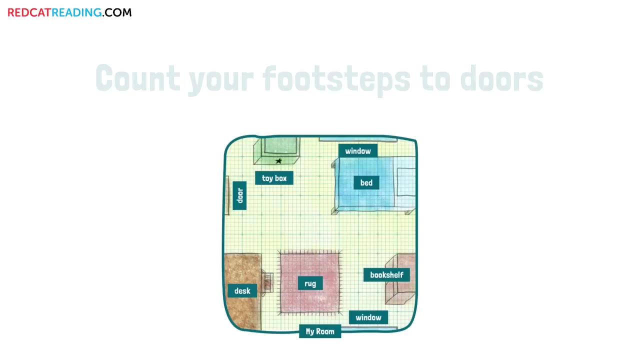 Draw the shape of the room Now. count the number of footsteps to different things. Draw those things in the room. Draw those things on your map. Add more things to your map. Count your footsteps to doors and windows too. Then color your map to look like the room.